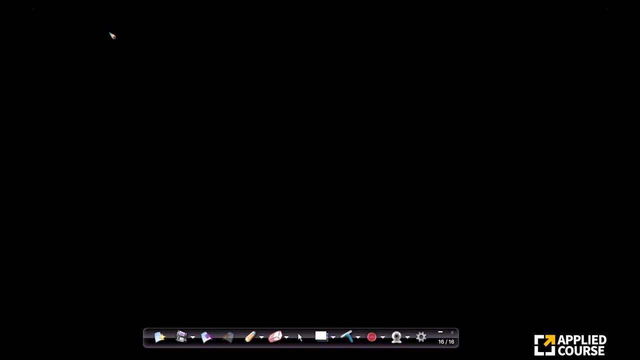 Now we want to solve this. Now let us go back to solving the recurrence relations. So I have: t of n equals to t of n minus 1 plus t of n minus 2 plus c. My favorite always is the recursion tree method because it is so visual and I can understand it better. Of course there are 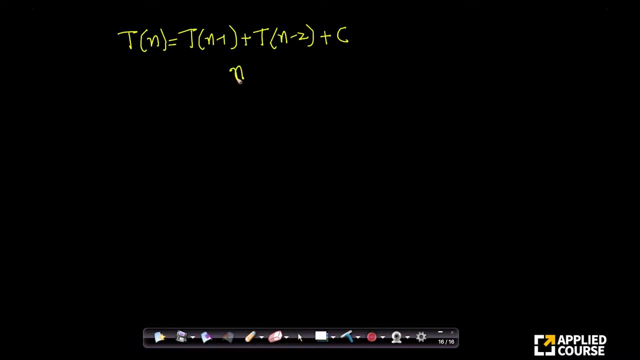 cases where master theorem and extended master theorem help, but this is my favorite. There are many ways of solving this. My favorite is always to draw because I can visually feel it. So problem of size n is broken down into problem of size n minus 1 and n minus 2, and to combine both of them. 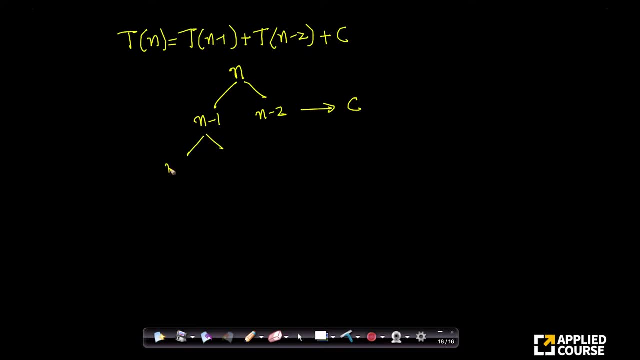 I need c operations. Again, this problem is broken down into n minus 2, n minus 3.. This is broken down into n minus 5 and n minus 6.. Right, So to combine both of them. again, I need c To combine. 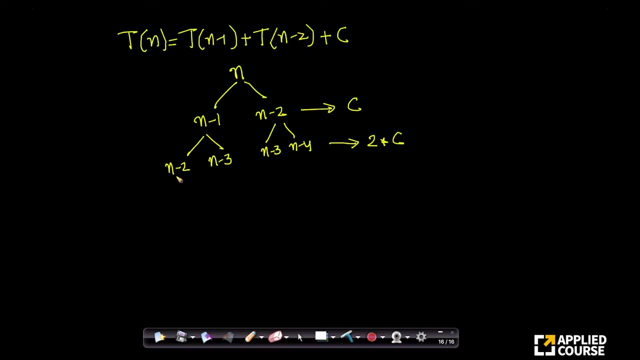 both of them again. I need c, So 2 into c. Now again, this will get broken up into n minus 3, n minus 4.. This will again get broken up to n minus 4, n minus 5.. Let me write it actually. 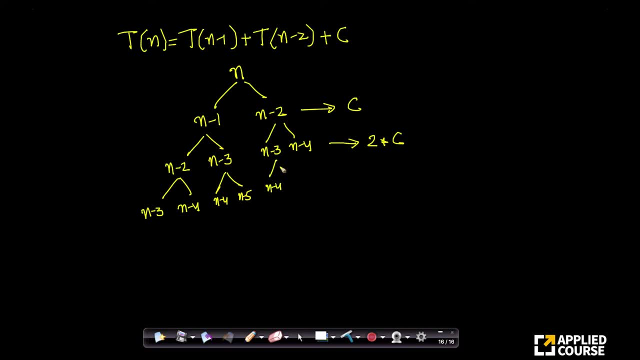 n minus 4, n minus 5.. This is again the same n minus 4, n minus 5.. This will get broken into n minus 5 and n minus 6.. Now I have 4.. I have this. I have this. 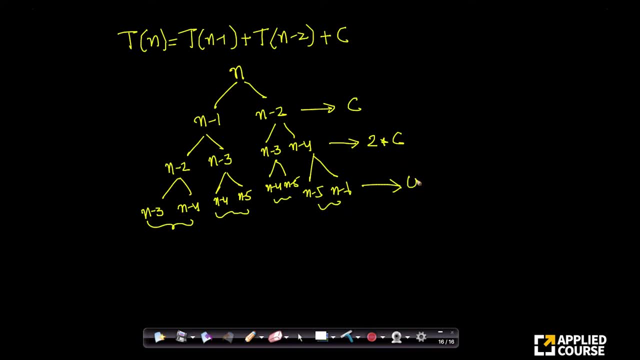 this. i have this that i need to combine. so i have four of them, four into c. you are seeing already the pattern. right, this is two square into c. again, each of them would get broken into two. right, each of them would get further broken down into two. so in the next level, what would i have? 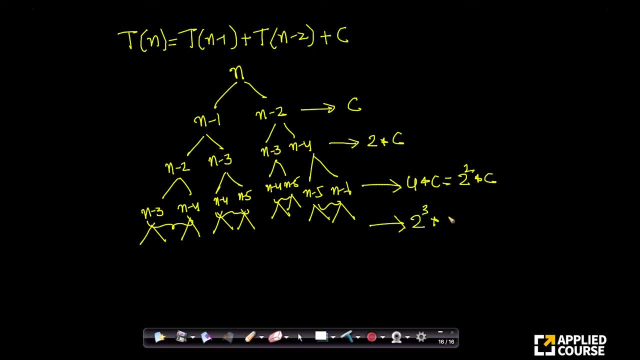 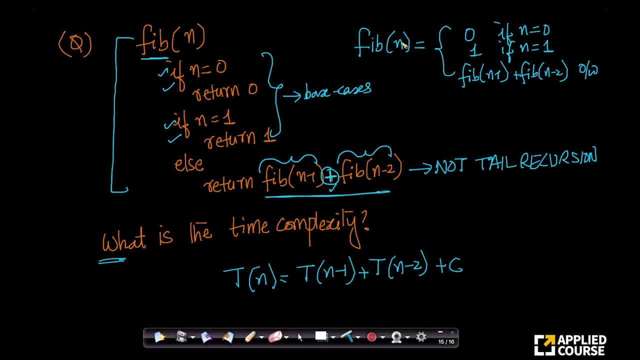 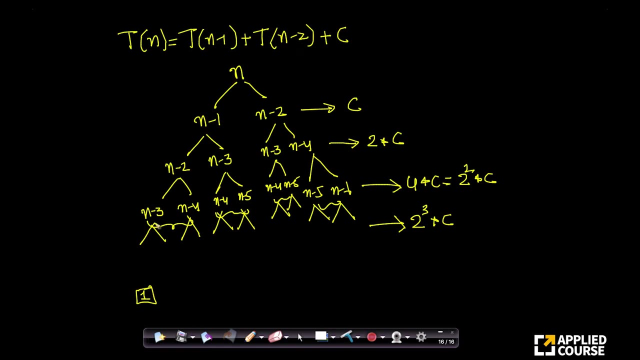 i have eight of them, right. i have two cube into c, so on, so forth, till the time i get one when i have only one element right, because if, when my n is equal to one, i know that i have to return one right. so, but look at this, the depth here, the depth of this tree here, the depth of the. 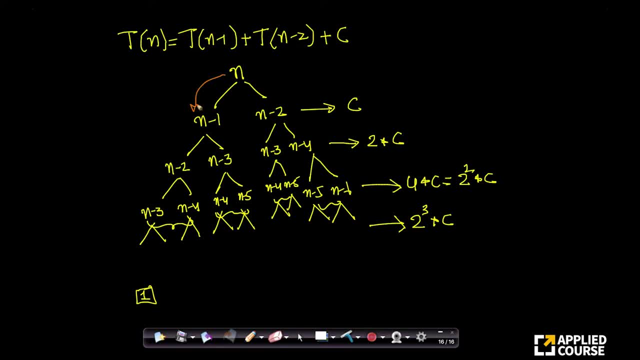 recursion tree: from n you're going to n minus one, to n minus two, to n minus three, so on, so forth, up to one on this side. on this side you are subtracting by two: n n minus two, n minus four, n minus six. here you will have n minus eight. so the tree on the right side is going to be shorter than. 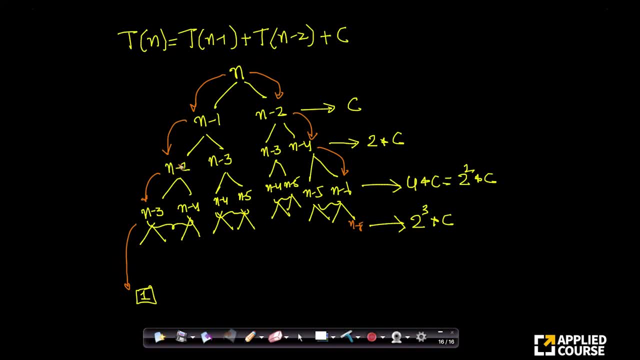 the tree on the left side. it's important to understand that. it may not hurt our analysis much, but it's important to actually say: all right, so sing to the left side, and then the next line, then the next line goes here. so g minus one does not mean g next. sometimes you will just previous. 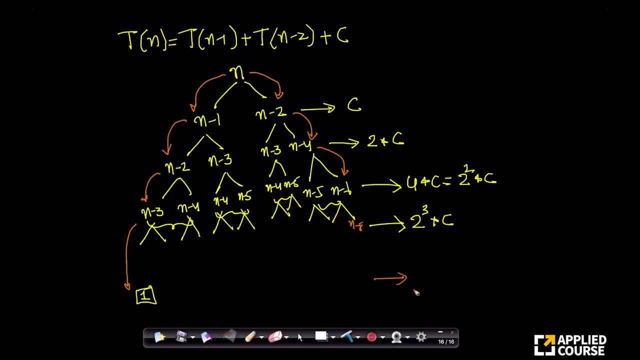 up and down that point. it is way more Harran, my all right del meina and one one, so left from here to understand. so there will be some. so in the last layer, okay. so this tree, this, this path, this path, this path on the right side is going to be slightly. 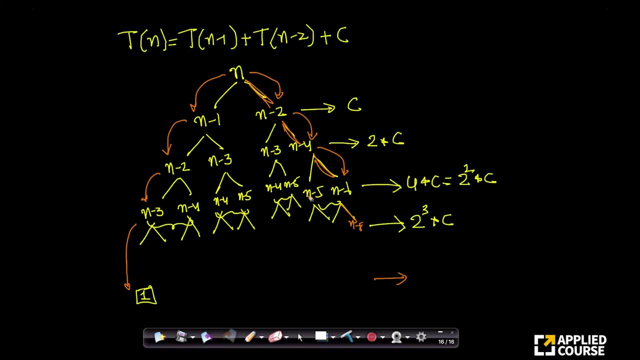 shorter. okay, not slightly, it's going to be shorter actually than the path on this side, right? that's because here you see, you are decrementing by 1, here you are decrementing by 2, so you will have some of them, right? for example, here you: 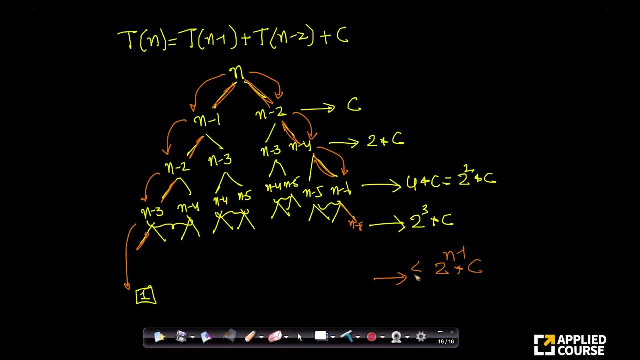 might have 2 power n minus 1 into C, you will have something less than equal to 2 power n minus 1 into C. you will not have exactly 2 power n minus 1 into C comparisons because some of these this paths would have terminated much earlier. 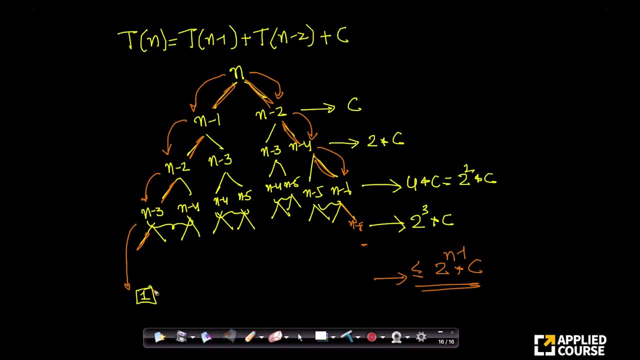 right. this path would have terminated probably here and while this path went on to here, right. so, in the time-complex analysis, because we want big O of something, we want an upper bound, right here. we are not looking for a tight bound, we are just looking for an upper bound. since we are looking for a upper, 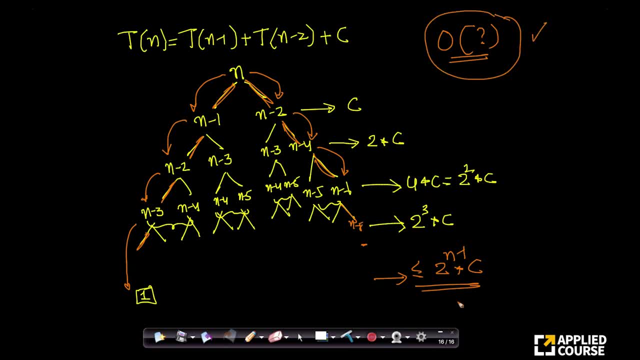 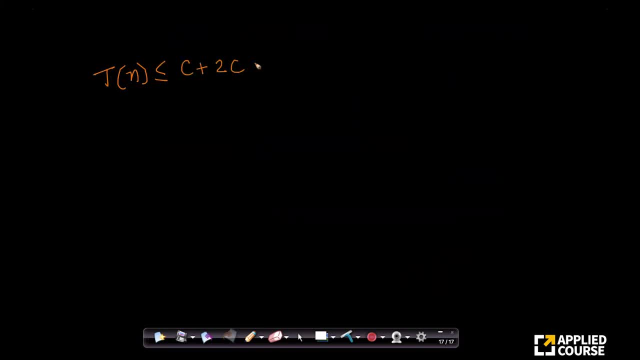 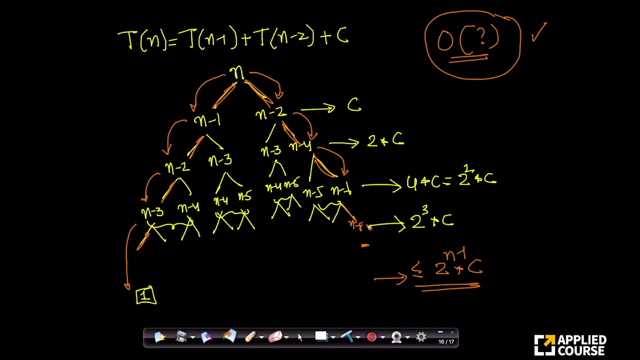 at C plus 2 C plus 2 square C plus 2 cube C, so on, so forth: 2 power n minus 1 C. but why did I put a less than equal to here? because because some of these, because this tree, this path would terminate earlier than this path. so in 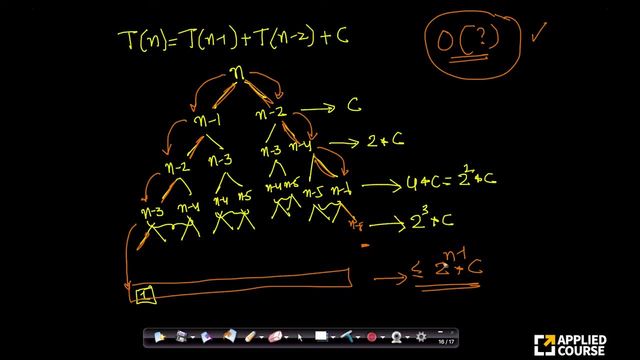 the last level. in the last level, I may not have these many, these many joints to take care of or these many combinations that I need to take care of. that's why I've written less than equal to here, but that's okay, because we want a upper. 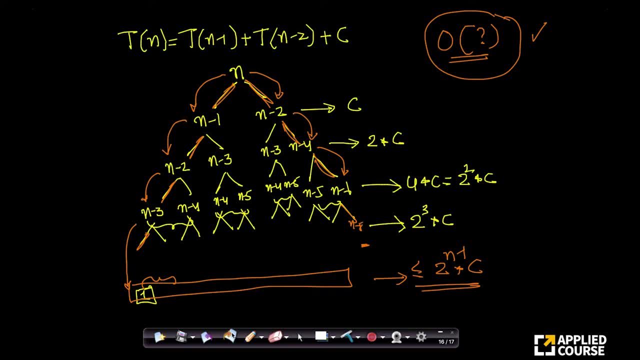 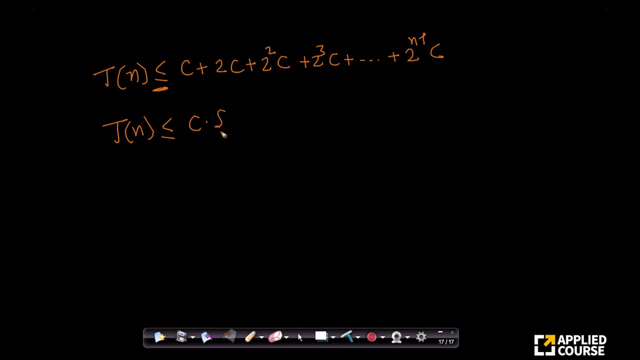 bound. we are not looking for a tight bound or a lower bound here. we're looking for an upper bound right. so what does this mean? this means my T of n is less than equal to some constant times right: 1 plus 2 plus 2 square, so on. so